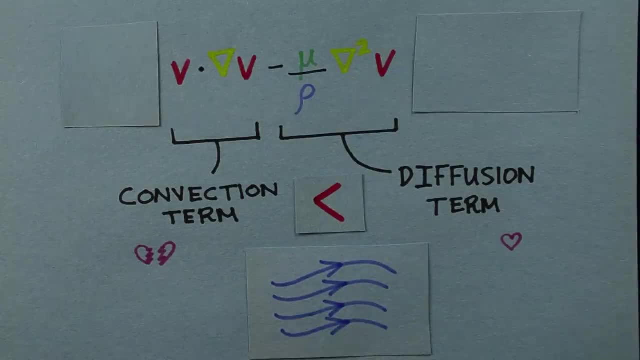 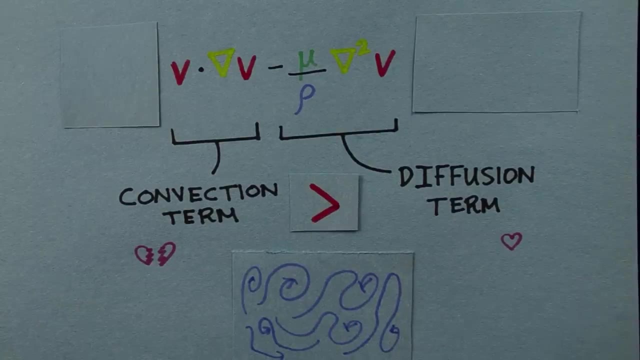 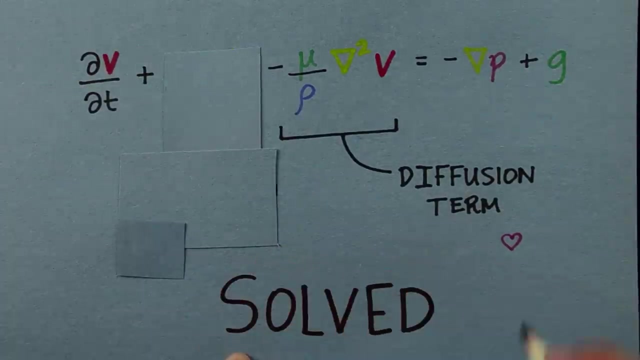 you get nice smooth flow, But when this guy is smaller than the other one, you get erratic, turbulent flow. This equation, therefore, is a constant push and pull between these two extremes. If we just deleted the bad term, we'd be able to solve the equation. 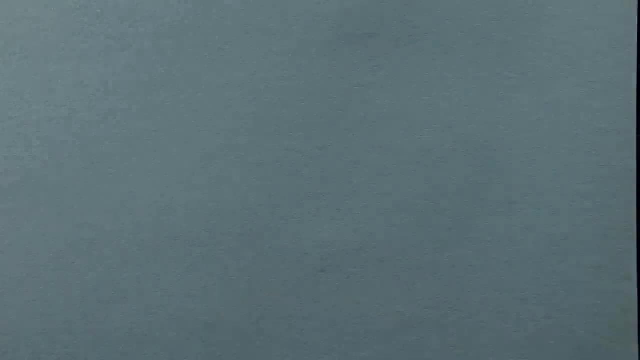 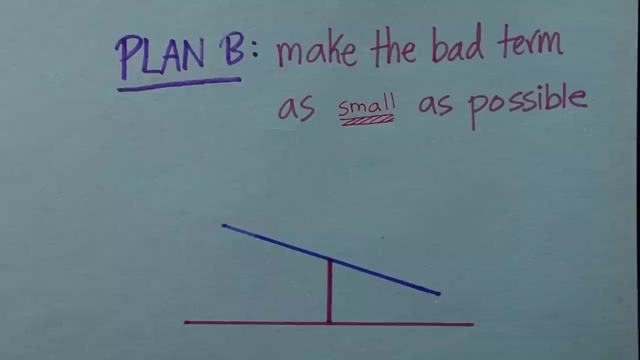 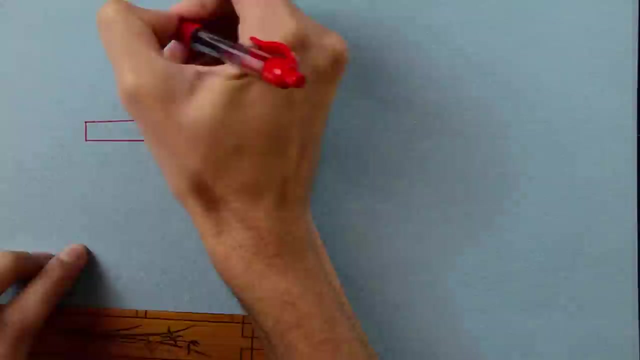 in minutes. Of course we can't just do that, But we can do the next best thing: Make the bad term as small as possible. That is, look at cases where the diffusion term is a lot bigger than the convection term, And there are two cases in which this would happen. One, if the fluid is very 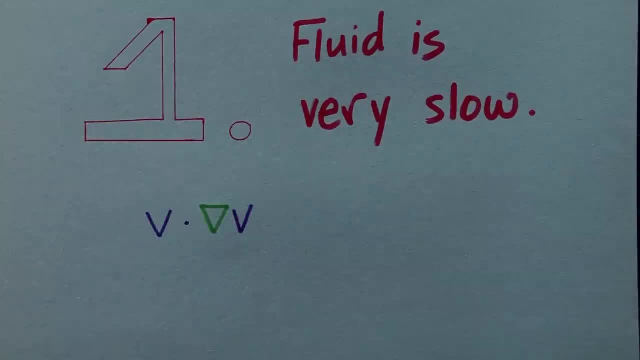 slow. Here, the velocity v would be very small, much less than one. So the convection term would be like v squared, which is much, much less than one. In this case, the good guy overwhelms the bad guy and we win. 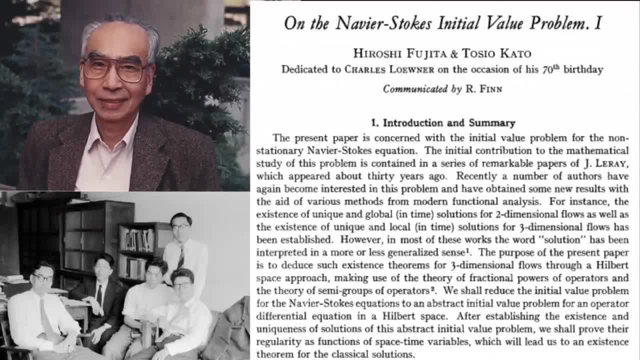 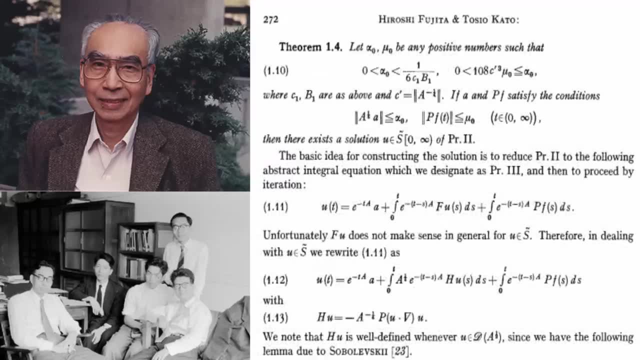 This was the result of a groundbreaking paper in 1964 by mathematicians Fujita and Kato from Japan. They proved that if you start off with a slow enough velocity field, then there exist smooth solutions to the Navier-Stokes equations. Now the definition of slow enough is quite technical. 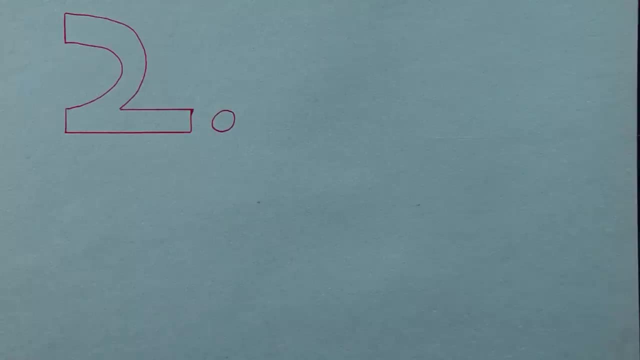 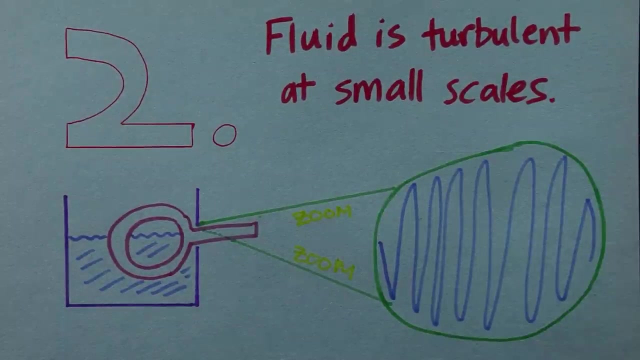 but that's what the paper says. 2. The fluid only has turbulence at a small scale, That is, you can only see the turbulence if you zoom in really close. What would we expect if we pressed play? Well, we'd expect all of these super. 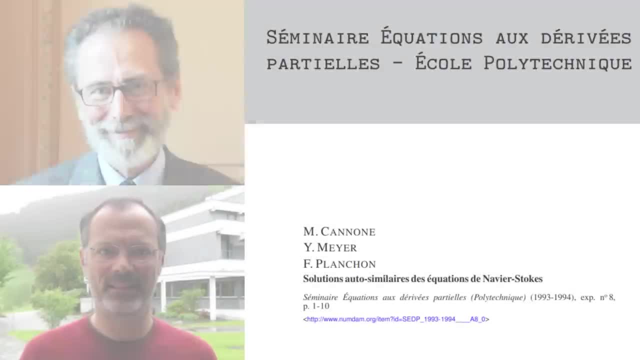 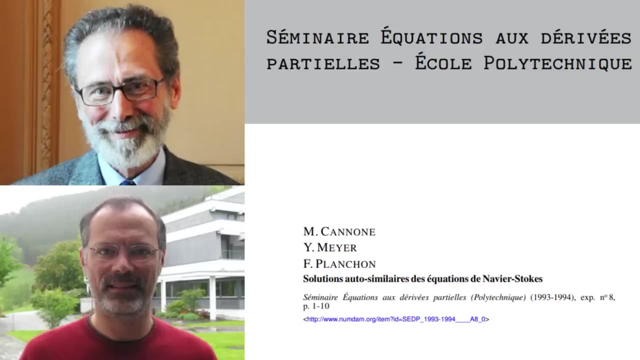 small wrinkles to even out. This was published 30 years later in a 1994 paper by these French mathematicians, whose names I wouldn't even try to pronounce. They proved that if your velocity field is very slow, then there is a lot of turbulence. at a small scale, That is, you can only see the 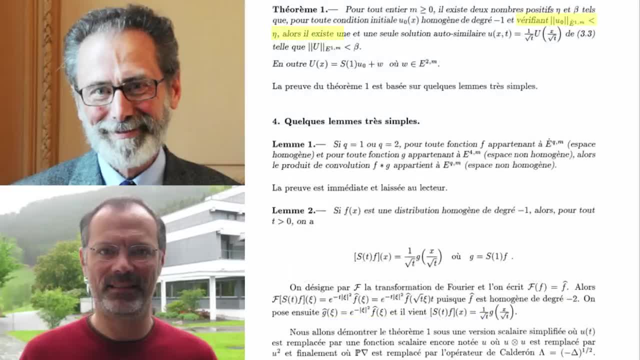 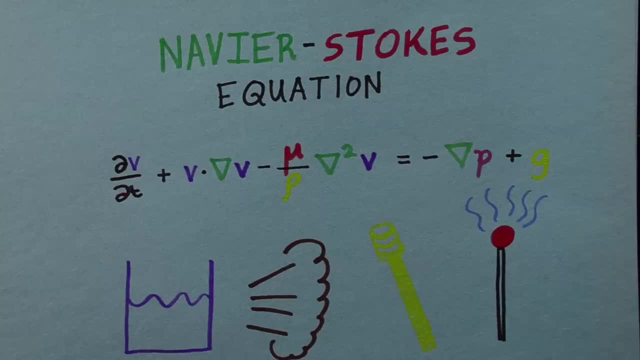 turbulence at a huge scale. But if the velocity field oscillates really fast, by a huge amount, the diffusion term dominates and we find smooth solutions to the Navier-Stokes equations. But this only deals with some special cases. we eventually have to confront the monster. 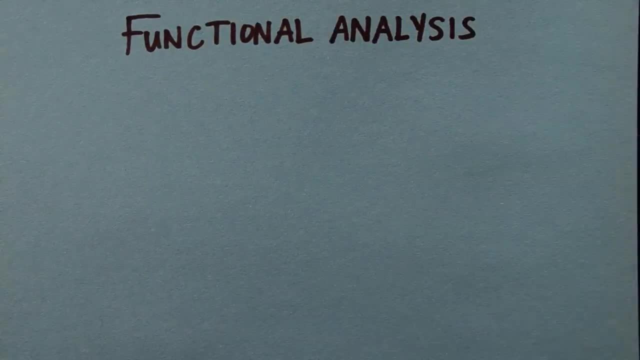 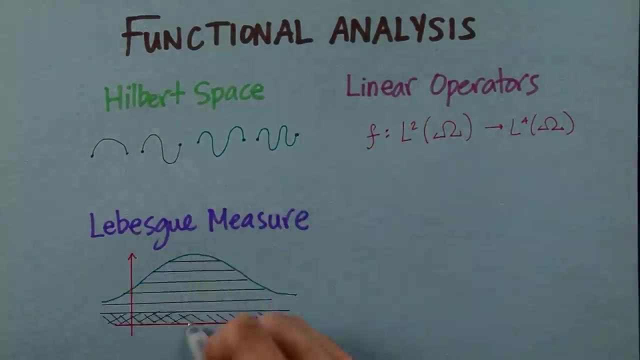 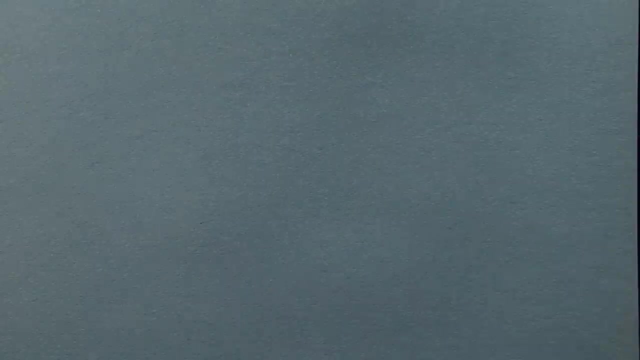 The main strategy people are using to do this is a branch of math called functional analysis. Here you study Hilbert, spaces, linear operators, Lebesgue, measure inner products, the whole deal. These tools allow you to compare functions with other functions. For example, we know what it means for a number to be bigger than another. 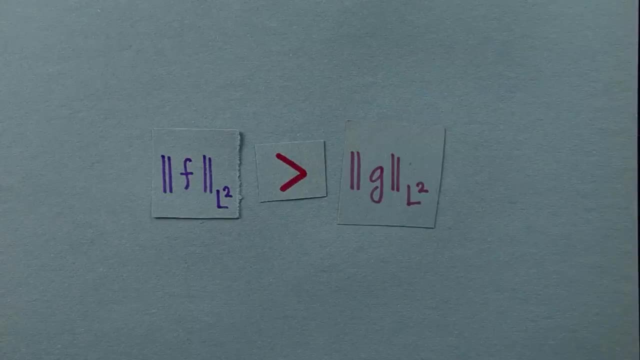 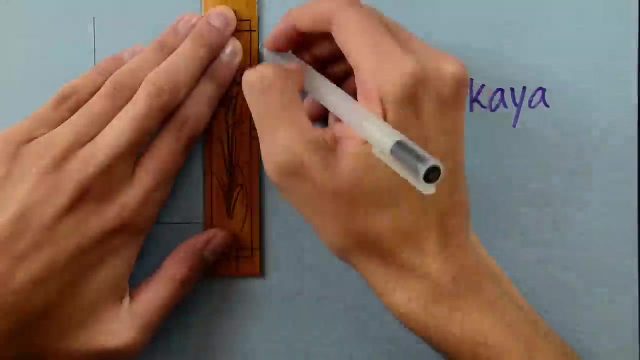 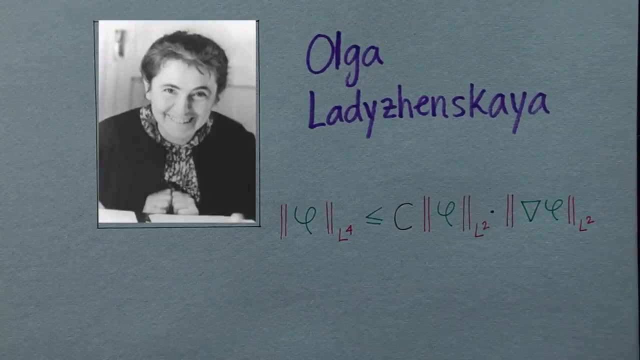 number. but what does it mean for a function to be bigger than another function? This is exactly what we need to gauge the size of the convection term. Mathematician Olga Ladishinskaya used a series of intricate inequalities to bound that term by a series of linear, simpler terms, The 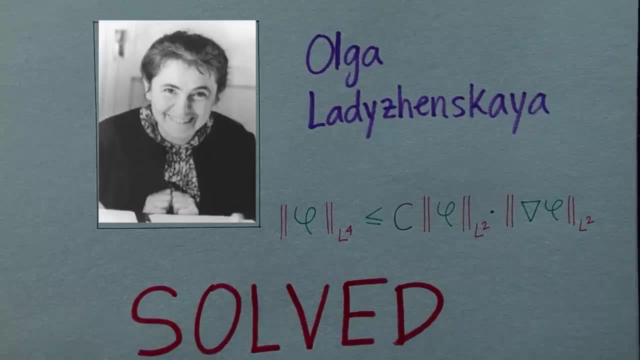 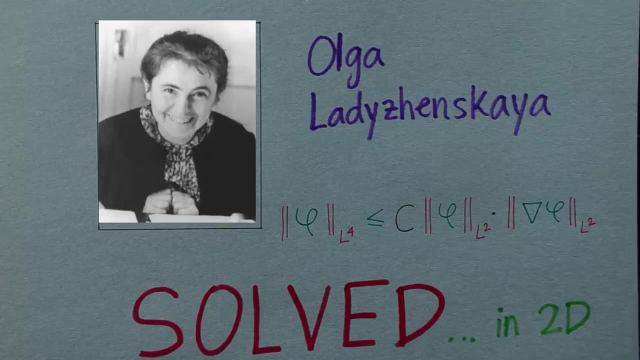 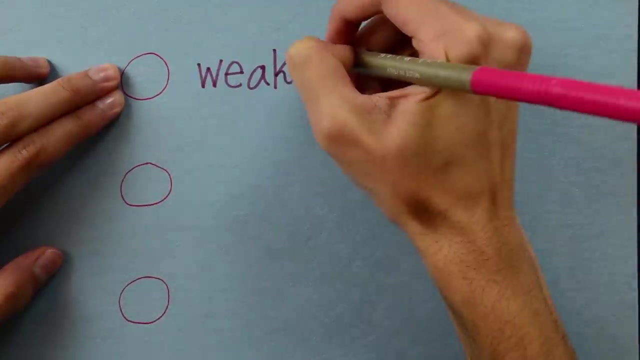 result was spectacular: The Navier-Stokes equations were solved in two dimensions. Unfortunately, the argument collapsed in three dimensions, so we were back to the drawing board. Since then, people have tried many other strategies. They've tried solving an easier version of the equation called the weak Navier-Stokes equation. They've tried using 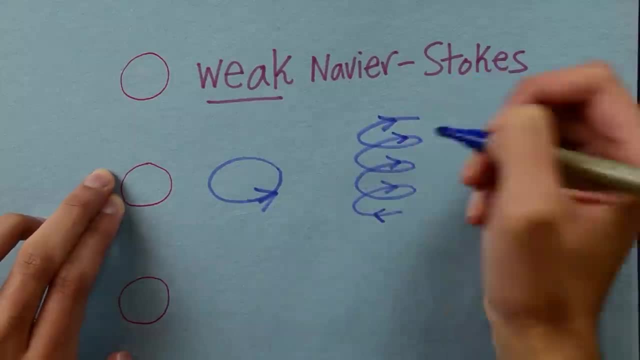 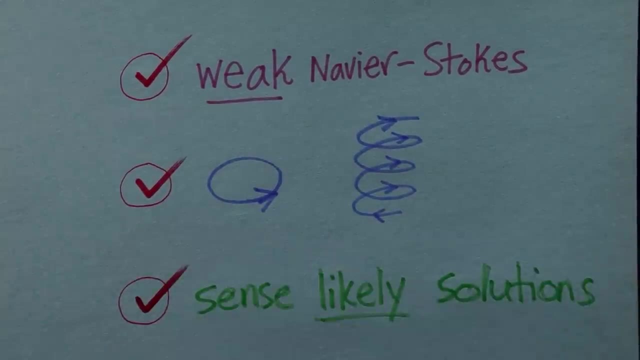 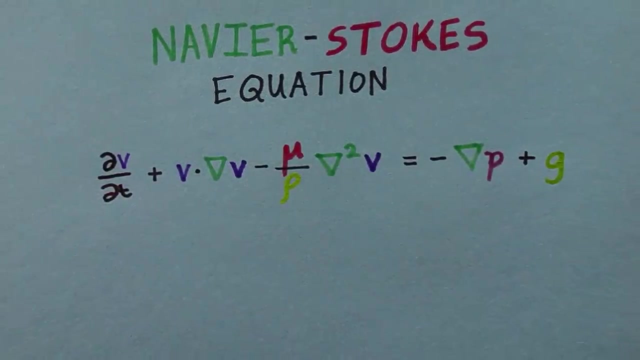 differential geometry to show that fluids traveling in certain paths have solutions. They've even tried using probability to guess likely solutions instead of the solution, But so far nothing has turned out correct. Now that we've seen the nitty-gritty of it, let's look at the big picture. 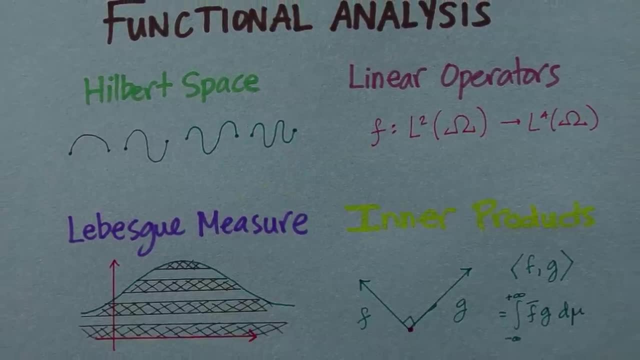 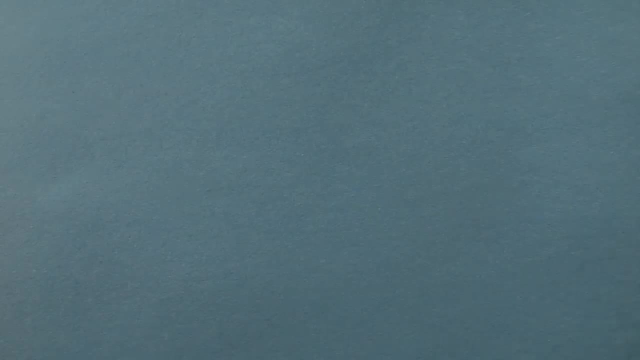 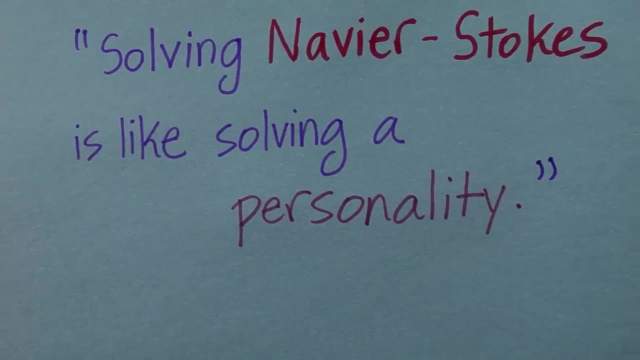 On one hand, we can think of this as just a math puzzle trying to solve an equation, but really it's something much more profound. My physics professor in second year put it like this: Solving Navier-Stokes is like solving someone's personality. This equation describes everything. 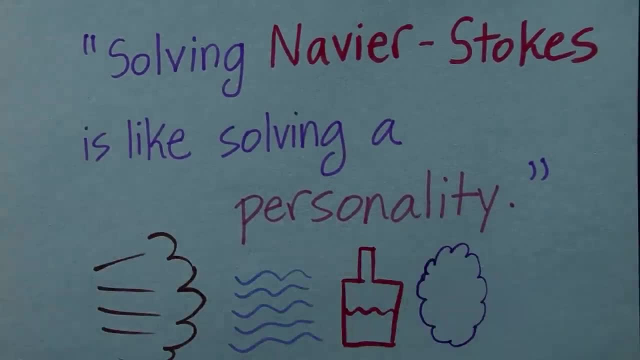 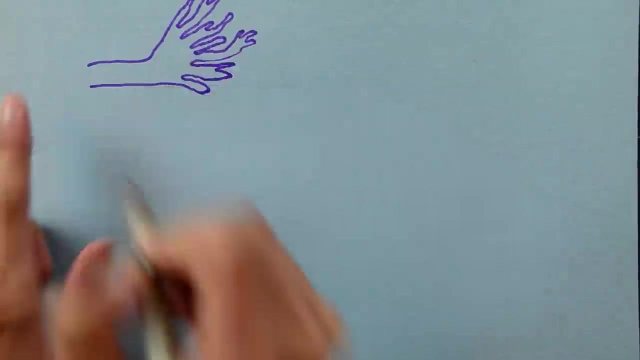 that flows Ever- Air, water, ketchup, gas, smoke- A solution to Navier-Stokes means that there is one and only one function that describes all of these things at once. This is nothing short of solving a personality. A personality is just a bundle of neurons and 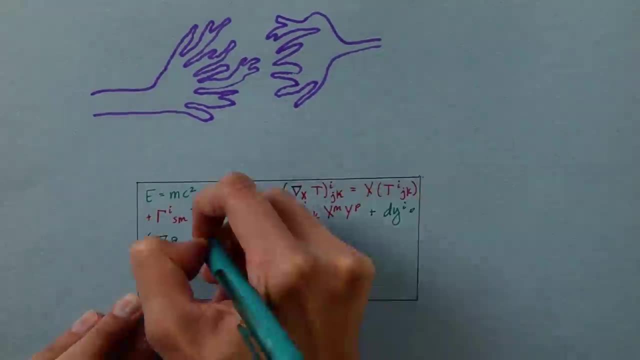 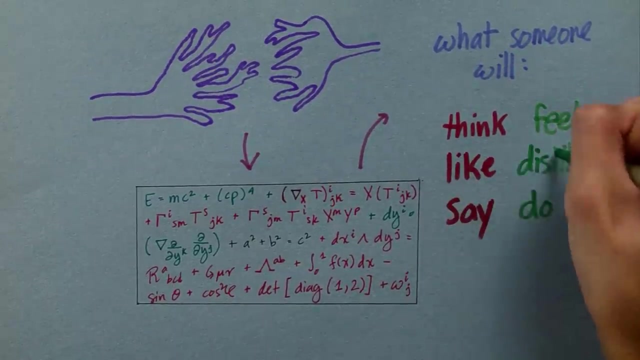 synapses in our brains. Could we put these connections in a gigantic equation which would determine exactly what someone will think and feel like and dislike, say and do at any given moment? Solving Navier-Stokes amounts to doing this. There's something. 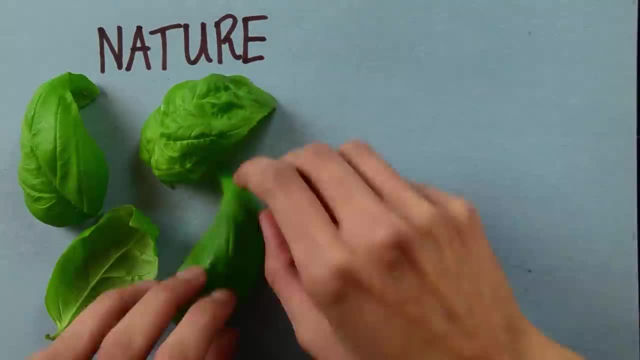 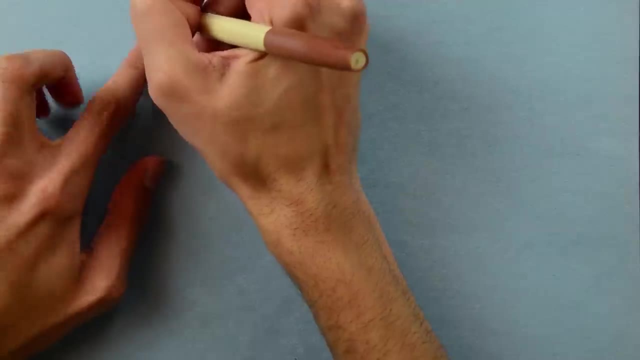 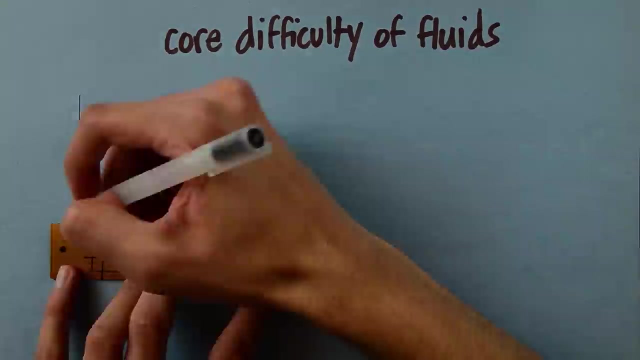 terrifying about that, About the fact that you can reduce nature to a clinical set of rules. But it goes beyond this. The core difficulty of solving fluids- their apparent randomness, their unpredictability, their chaos- is common to so many things. For example, how stock markets